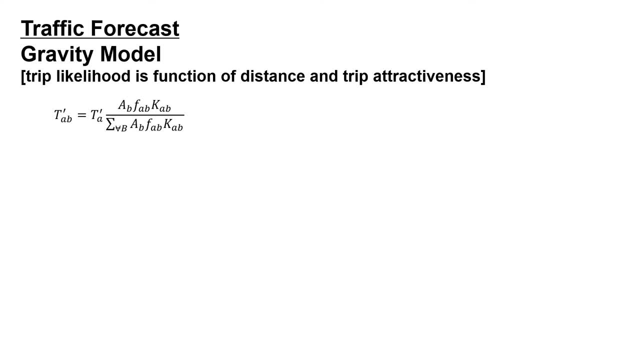 And the underlying assumption is that the likelihood that a trip occurs is a function of the distance and the trip attractiveness, and so that's what we're going to use this equation for. Of course, there's many more sophisticated models in traffic forecasting. This is a simplified model just looking at this one perspective, but there are lots of other things that we can consider if we were actually doing traffic forecasting. 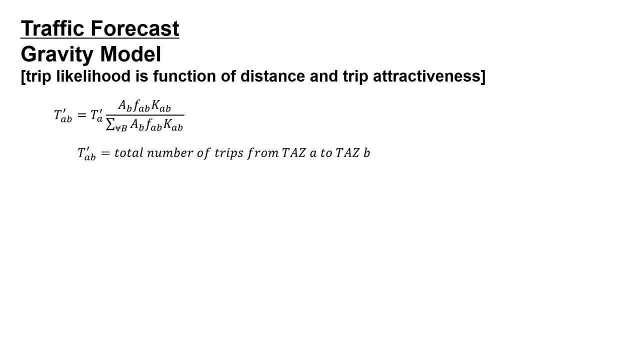 And so what we're going to do is we're going to solve for the total number of trips from TAZA to TAZA, And where TAZ is the traffic analysis zone, and so this is what we're going to use the equation for. So we're going to start with the total number of trips from TAZA. so how many trips does TAZA produce? and we're going to look at distributing it and essentially, we're going to weight this by the other zones and factors for the other zones, and those factors are the total number of trips attracted from TAZB, the distance or the travel cost, and this is what we're going to use the equation for. 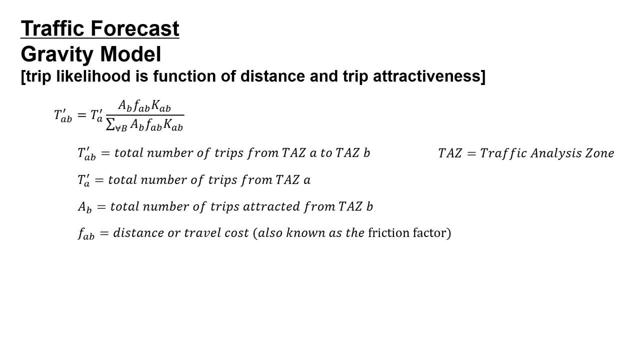 And this is also known as the friction factor, and a lot of times the value we use for that is one over the travel time from zone A to B. And then we have a socioeconomic factor, a parameter that is going to help us balance the results, and what it's doing is helping us measure the relationship and the likelihood between these two zones, A and B. 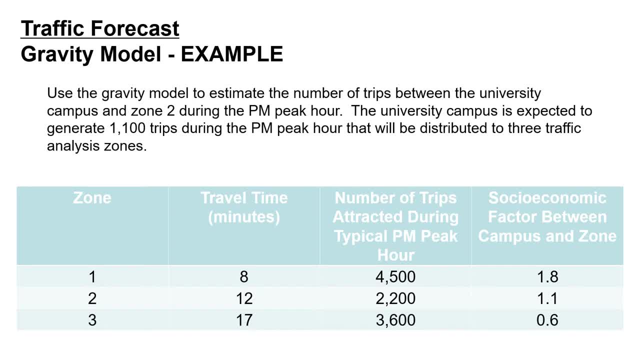 So we're going to take a look at an example. We're told we should use the gravity model to estimate the number of trips between a university campus and zone 2 during the PM peak hour. The university campus is expected to generate 1,100 trips during the PM peak hour and it will be distributed to these three traffic analysis zones. Of course, this is a very simplified example. In reality this would be much more complex and labor-intensive. but we're looking at a few zones here. 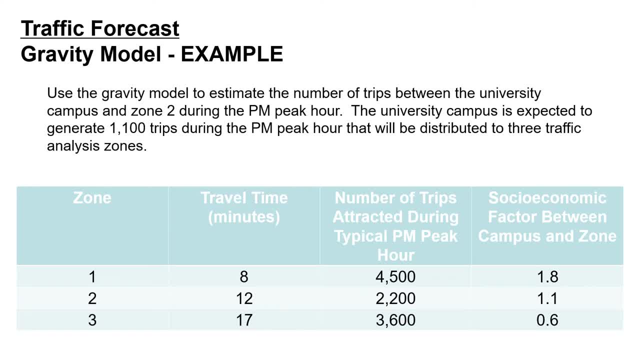 So we have some data on each zone and we're going to start with the first one, which is the distilled traffic in the zone B. So the data we're going to put together is the effect of this. We've got the travel time in minutes. We've got the number of trips attracted. 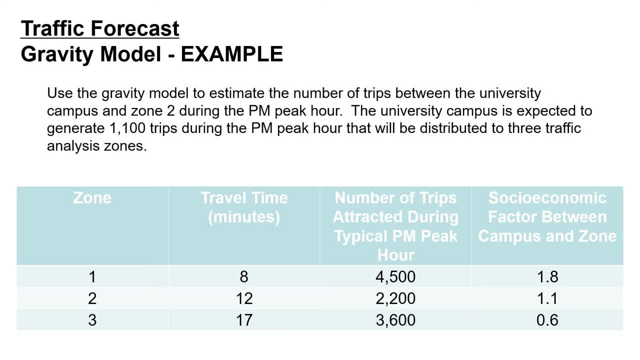 during a typical pm peak hour. That doesn't mean from our zone in particular. It's just that's what these zones are attracting during the pm peak hour and this is gonna help us give us an idea of how we're gonna. it's gonna influence how. 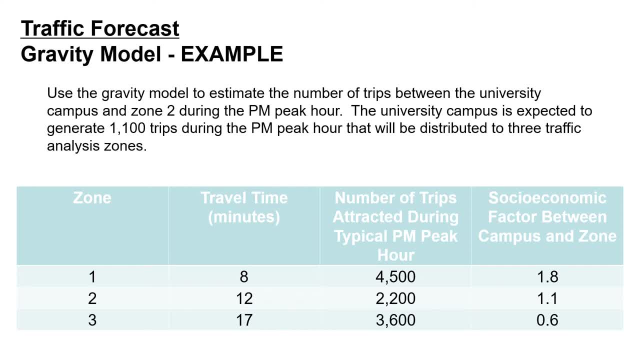 those 1,100 trips from our campus are gonna be distributed. And then, finally, there's a socio-economic factor between the campus and each zone, and the higher that that value is, the higher that factor is, the more relationship there is. And so, for instance, if we're thinking about it in the context of a 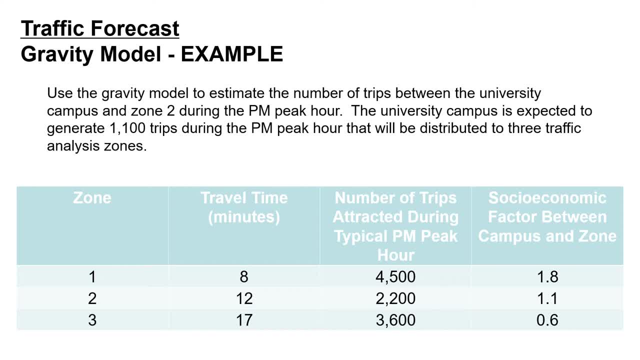 university campus and how we're gonna distribute those trips. those would be things like: are there housing? are there affordable housing for college students? And so the higher that factor is, that's telling us there's there's a strong relationship between the these two zones- campus and the zone- and that there's 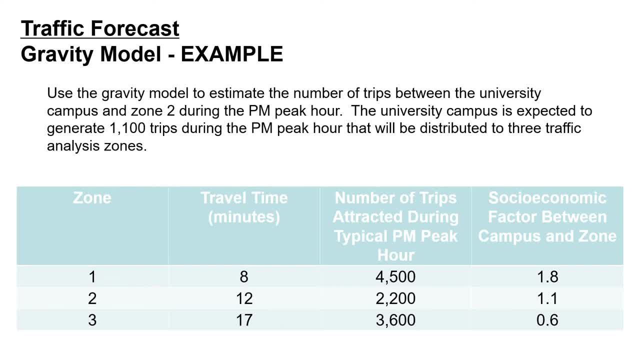 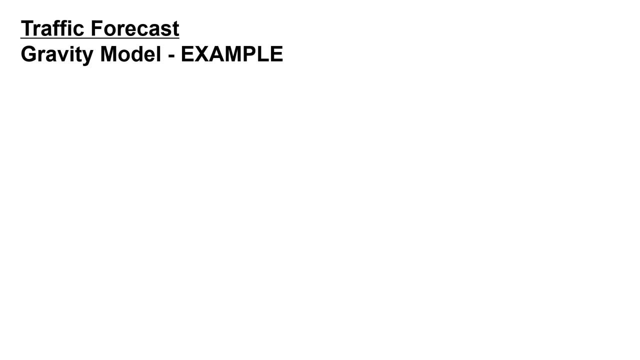 housing opportunities there or there's attractions that they would be, they would want to travel to, And lower values represent lower likelihood or lower relationship between those, the campus and that zone. So we're going to start by setting up our table here, one row for each zone, and 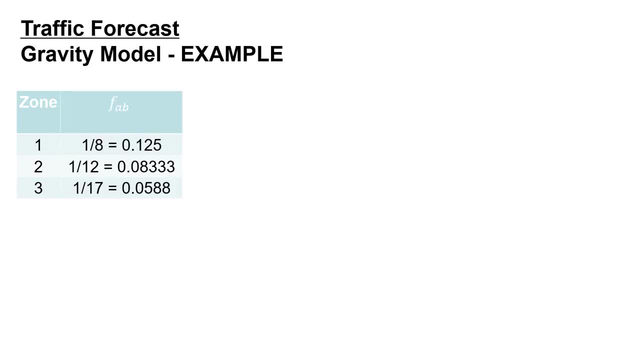 we're going to start with our friction factor F sub a, B, so the friction factor between zones A and B, And, as I mentioned, it's typically the inverse of the travel time. So for zone one it's one divided by eight, which gives us a. 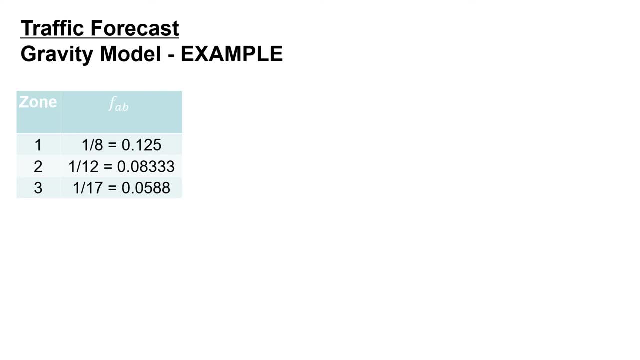 friction factor of 0.125. and then the next one is 1 divided by 12, and then 1 divided by 17, for Zones 2 and 3.. For our attractions, this just comes the trips attracted to TAZ B. This is our given, so 4,500 for Zone 1,, 2,200 for Zone 2, and 3,600,. 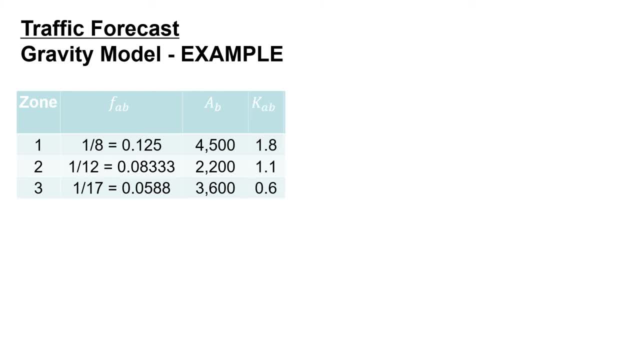 2 and 3600 for zone 3. now we have our socio-economic factor and this is going to help us balance the results and it also gives us the relationship between the two zones of interest. so the higher that socio-economic factor, the more similarities there are in the more likely, the higher the likelihood that 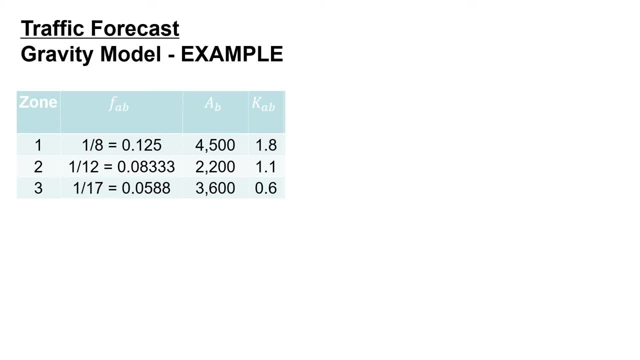 they are related. so, for instance, this 1.8 in this example could mean that there's more housing for university students, and so there's more likely to have that connection, where zone 3, with the lowest number of the value of 0.6, means that there's less similar socio-economic factor. so there's likely. 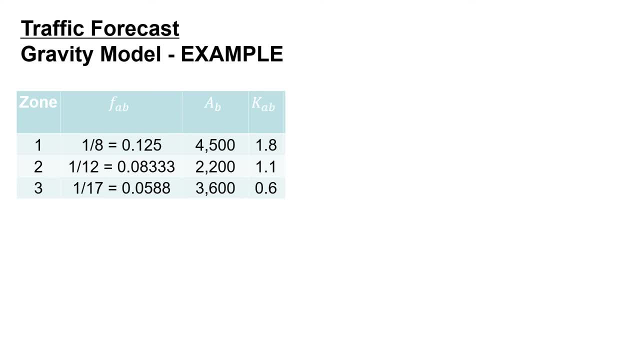 going to be less desire for travel between those zones. our next column is to multiply those three values. so for the first row, we would multiply point one to five times forty, five hundred times one point eight to get a value of 1,012.5.. We're going to need to sum up this column. We get a summation of 1,387.177.. 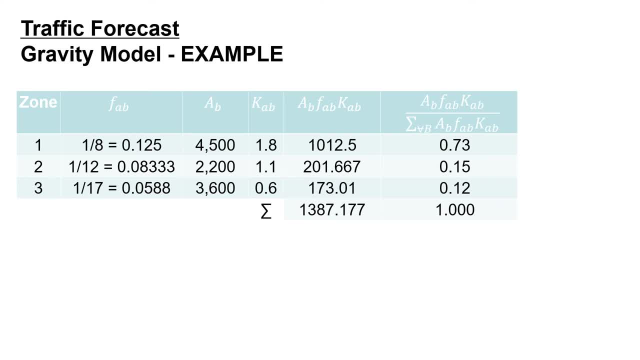 And then, basically, we're going to use this column and that total to distribute the trips, our 1,100 trips. So in this next column here we're going to take each individual value from the previous column and divide by the total. So start with the first one: 1,012.5 divided by. 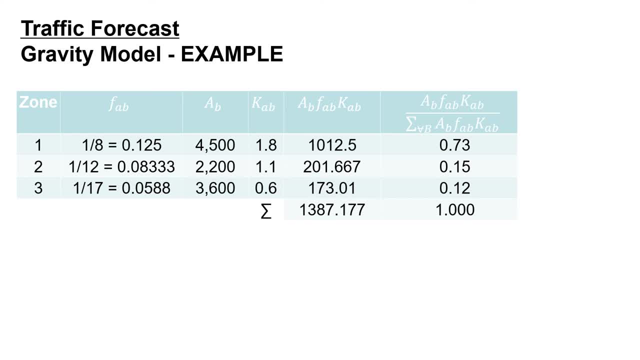 1,387.177.. And that's going to give us our value of 0.73.. So again, we're going to take this value divided by 1,387.. And that's going to give us 0.73.. 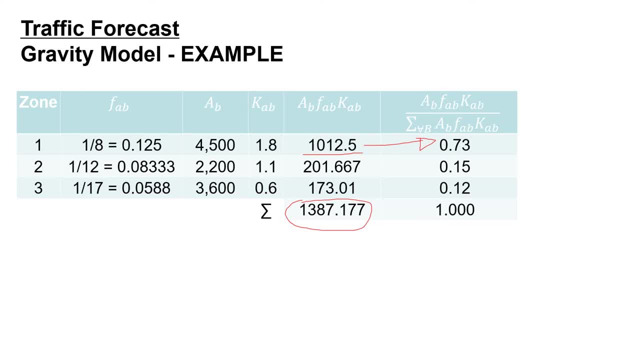 We'll do the same thing for the next row. This 0.15 is equal to 201.667 divided by 1,387.177.. And this is telling us roughly that we're going to have 73% of the trips go to. 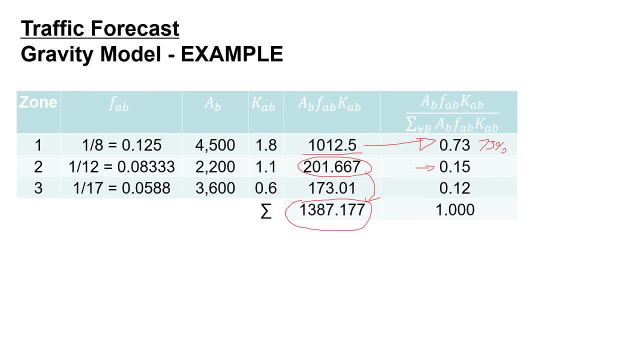 or attributed to zone 1,, 15% in zone 2, and 12% attributed to zone 3.. And that should sum up to 1.. So again, the previous steps, ultimately, are just helping us apportion what amount is going to go or be attributed to each zone. 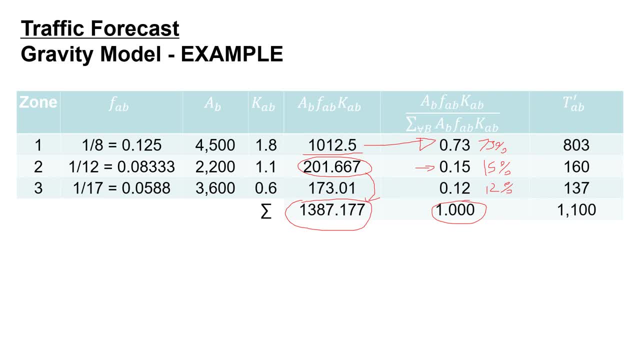 And for our actual trips we're going to multiply those percentages or those portion proportions by 1,100.. So we'll have 803 for zone 1, 160 for zone 2, and 137 for zone 3.. Our question actually asks us about the number of trips between the university campus and zone 2 during the pm peak hour.